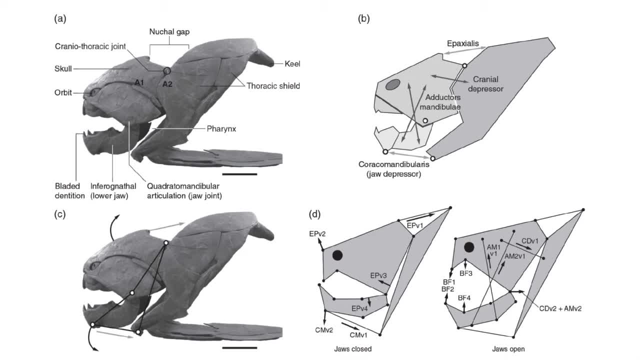 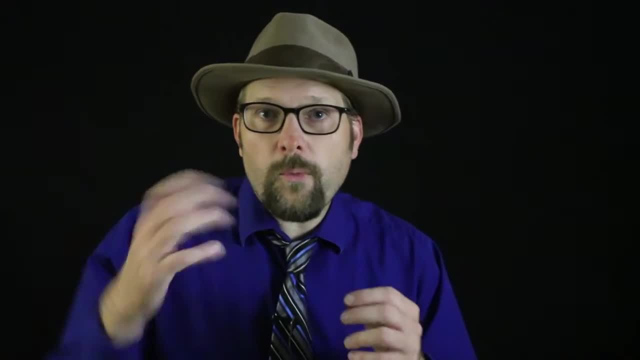 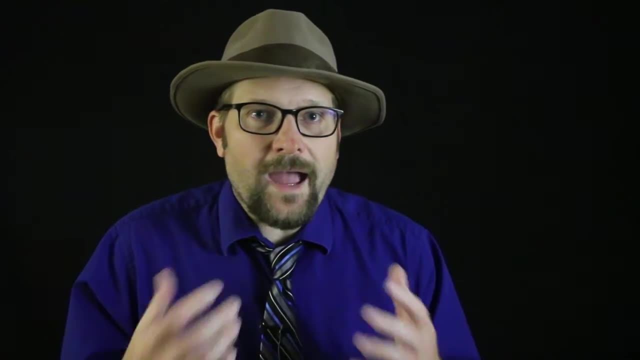 the head to move up and down, while also exhibiting a strong jaw joint. This arrangement provided a very quick motion For both opening and closing the jaw and allowing a really strong bite. These fish were active predators who fed on any fish, whether they were armored or not. 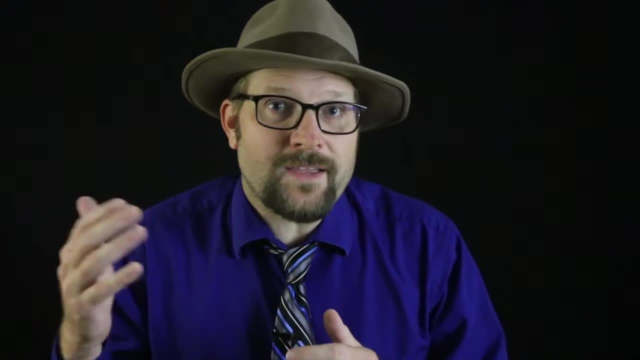 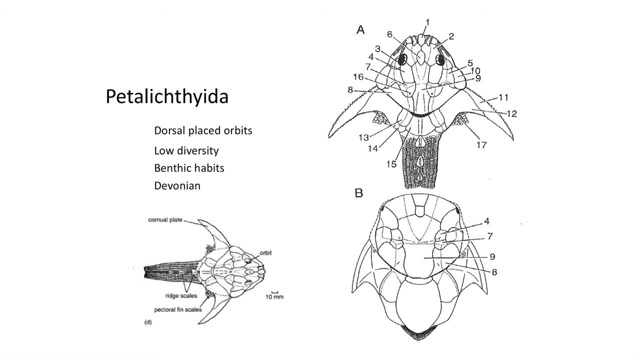 The Arthiidae also exhibit live birth rather than having eggs, a feature found in some sharks and bony fish. The next group are the Peliichthya, a less diverse group of fish that live during the Devonian. 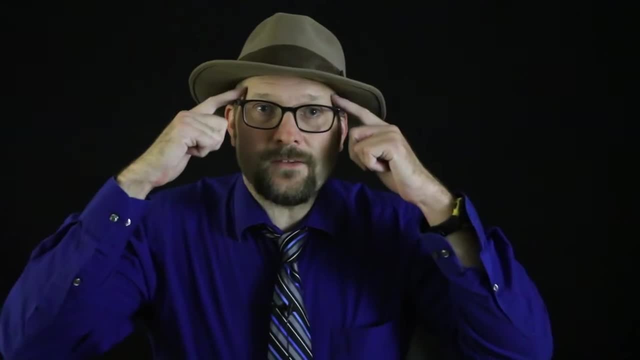 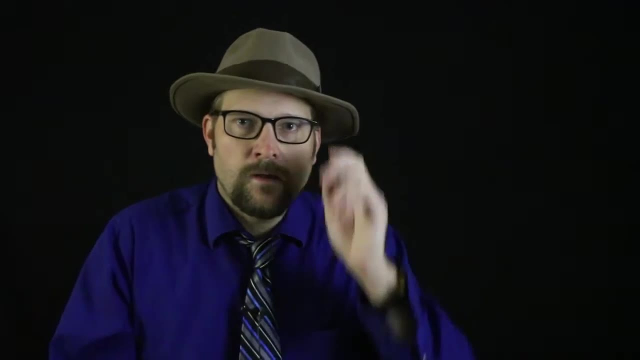 With their low weight they are more likely to die With wide heads and eye sockets opening upward. these fish are thought to be benthic living swimming near the ocean floor. The Tychiodontid are well known, primarily from their tooth plates. 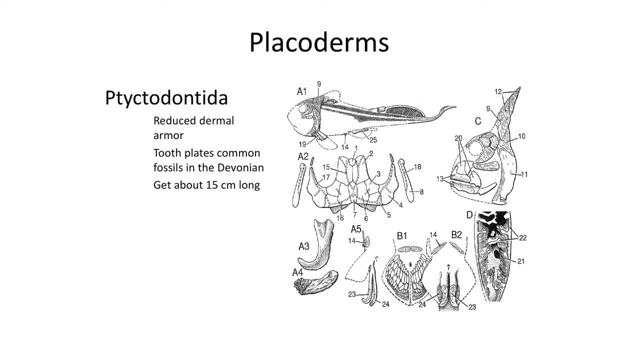 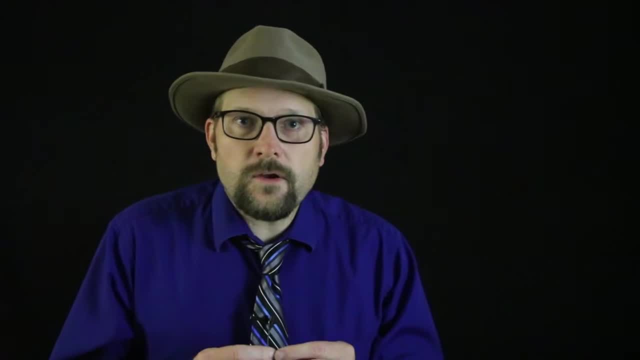 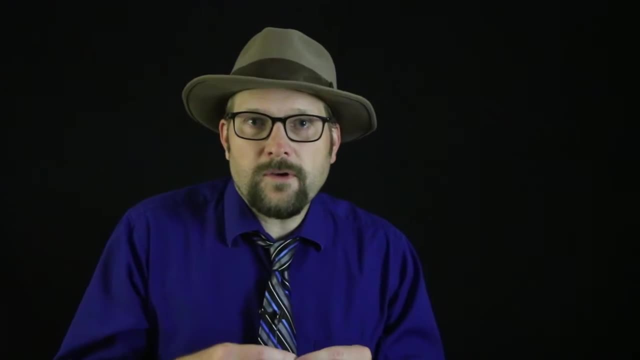 These less armored fish exhibit claspers in male individuals. Claspers are a feature seen in Chondrichthyans such as sharks. they are used for internal fertilization of eggs. These claspers are believed to have maybe a rose, independently than those found in sharks. 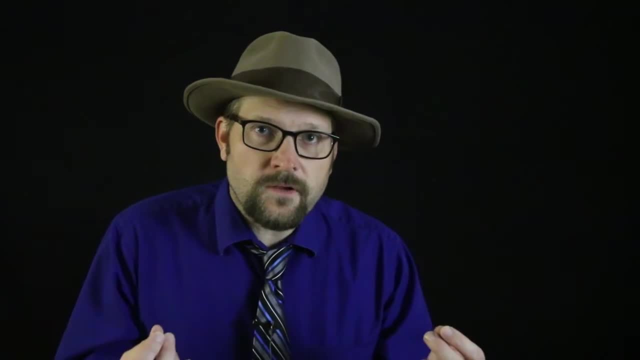 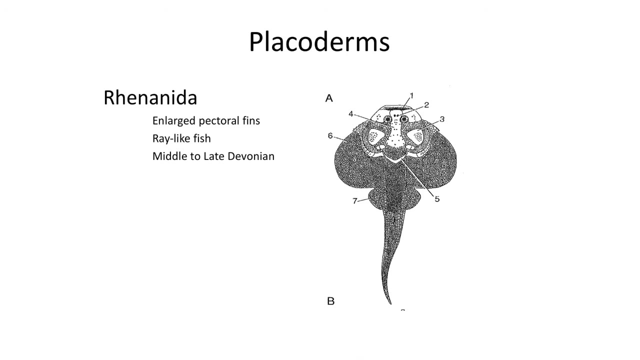 but there are other similarities between Plachioderms and sharks to suggest a close relationship between the two groups. The Rhaenidae are very ray-like Plachioderms with large pectoral fins and a very flat body plan. 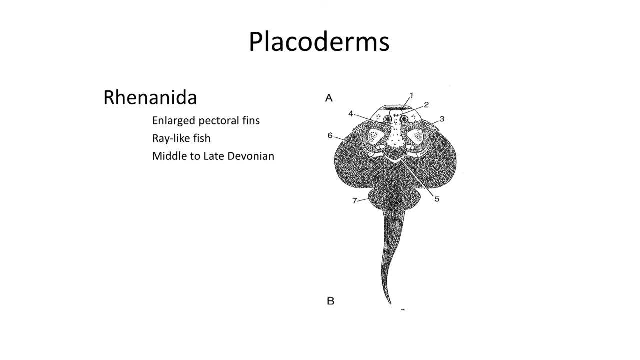 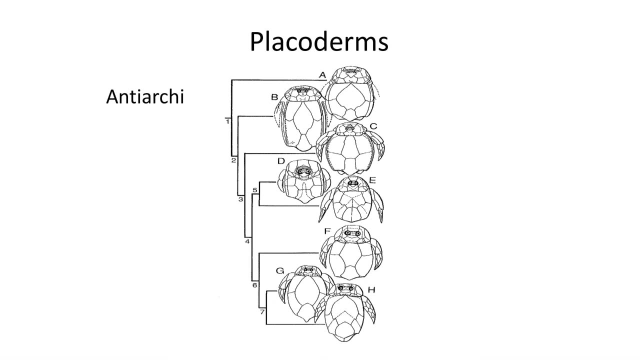 These are known from the Middle to Late Devonian. They have occupied the same niches as modern rays do today. The last group are the Anarchaea, one of the most successful groups of Plachioderm fish living during the Devonian. 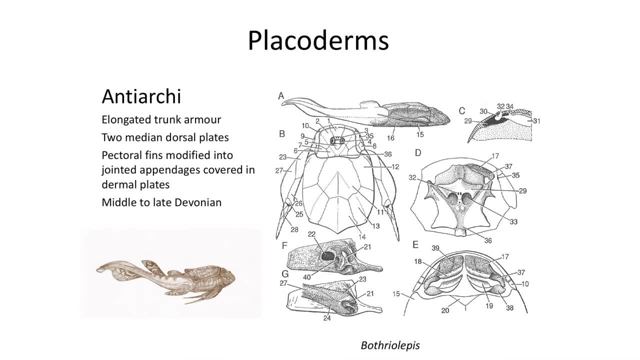 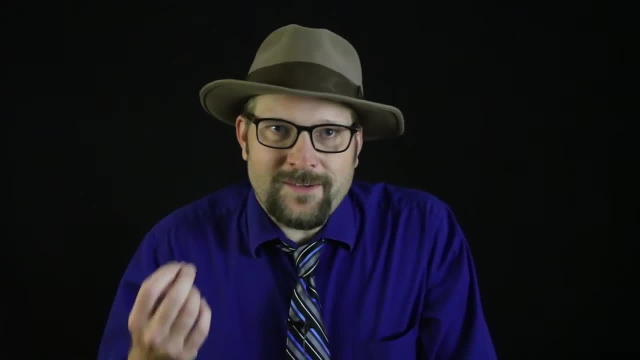 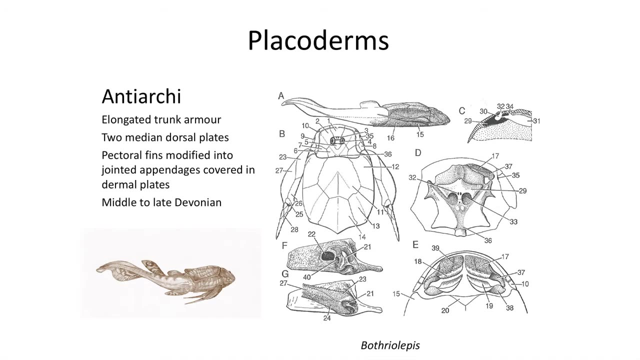 These fish are weird in having armored their pectoral fins, which are encased in bony plates, a little like armor found in medieval knights. The top of the head was covered in two dorsal plates With eyes positioned close together. one of the most well-known Anarchaean fish is Bothylepis. 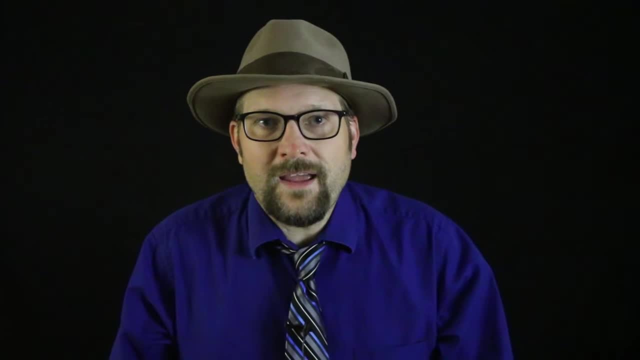 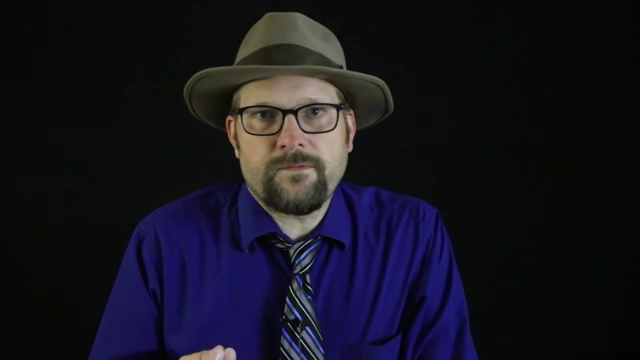 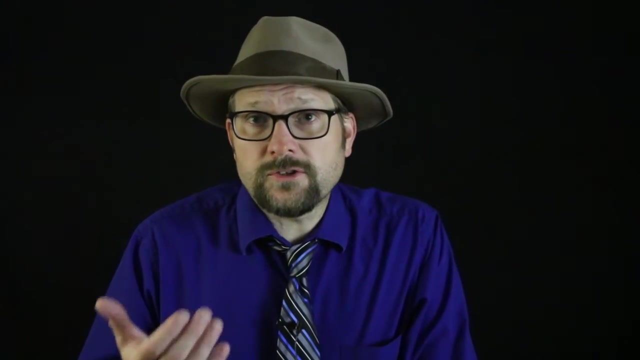 which is known from the well-preserved fossils from New York and have been found from many Devonian sites around the world. Aside from these armored Plachioderm fish, there was an array of other early jawed fish, most of which are closely related to modern sharks. 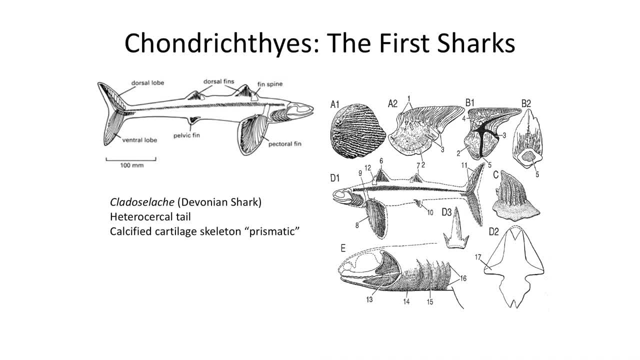 The first Chondrichthyans, Cletus Sleekiae, are known for their long-tailed fins and their long-tailed fins are known for their long-tailed fins. They are also known for their long-tailed fins. The second Chondrichthyan is known from the early Devonian, which closely resembles a. 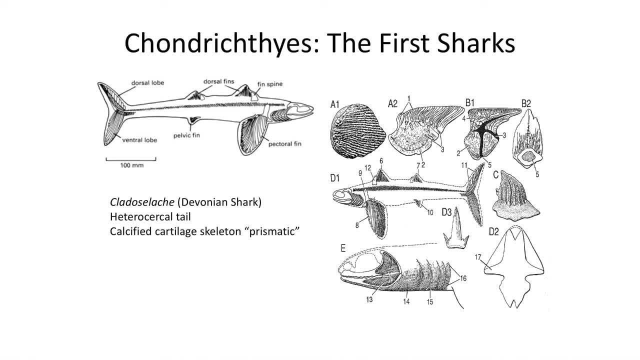 modern shark. The skeleton was made out of cartilage and features a large pectoral fin. The fossil is an impression, since only the teeth and scales of these less armored fish survive fossilization. After the Devonian, the Chondrichthyans, sharks, rays and chimarids really started to diversify. 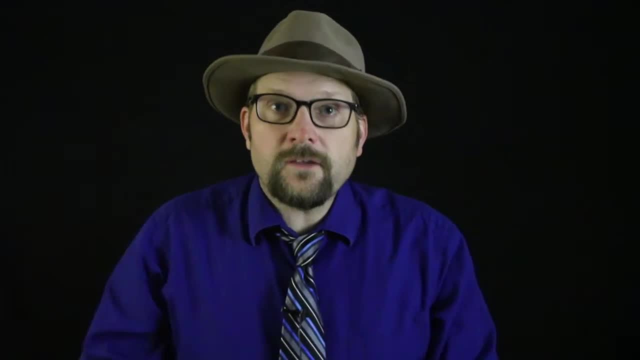 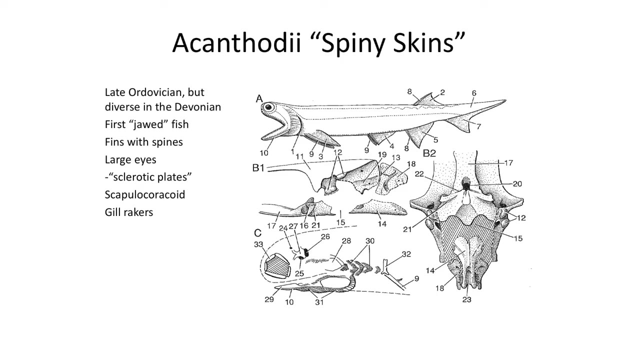 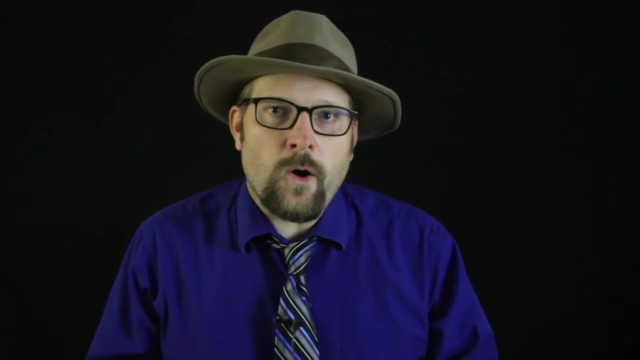 and we will talk about their evolution later on. Now In the Chondrichthyan there was another group of early fish which lacked armor: the numerous Ancanthodian fish. These are also known as the Spiny Skins. Now there is considerable debate right now over the relationship between Ancanthodian 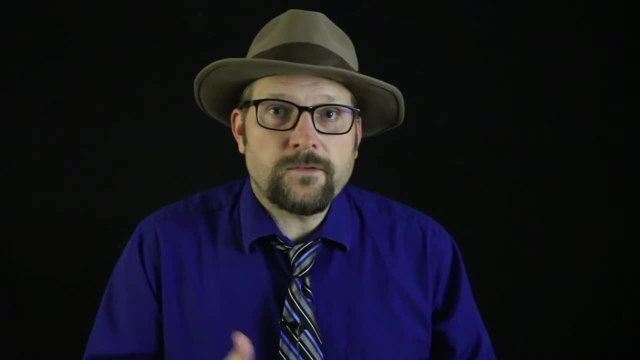 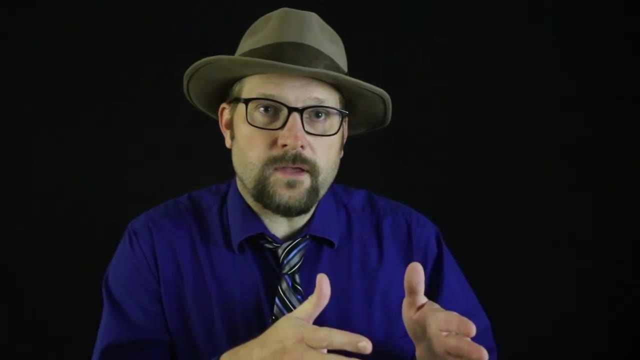 fish with both Chondrichthyans as well as the bony fish Osteoichthys. Some researchers place the Spiny Skins in with the Chondrichthyans, while others place some of the spiny skin fish within the bony fish. 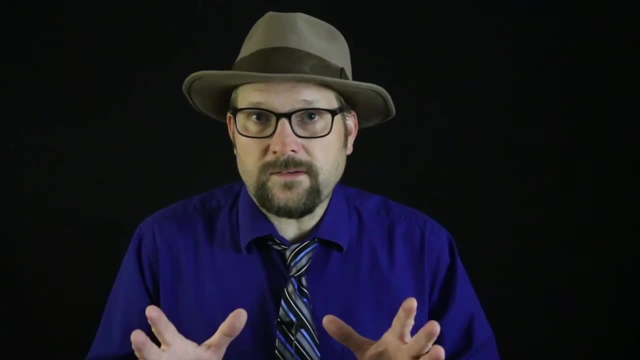 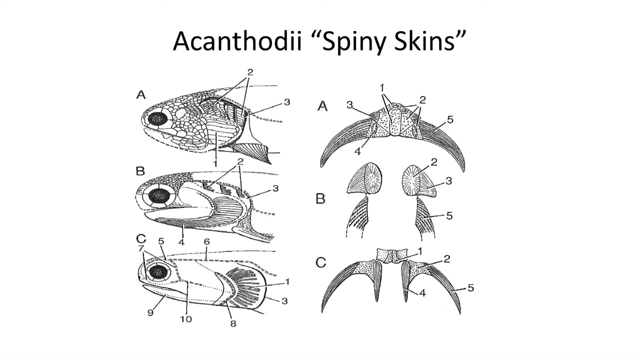 Now there are a couple of interesting features in spiny skins that make them more advanced than fish we've seen before. Ancanthodians have a scapular coracoid, which is a bone that supports the pectoral fin spine. 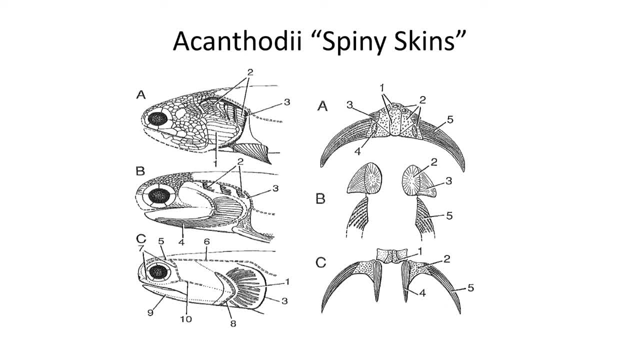 The group show a diversity of fin spines that protect them from predators but allow them to be more nimble and quicker in their prey. This is an interesting feature of the fish: that protect them from predators but allow them to be more nimble and quicker in their prey. 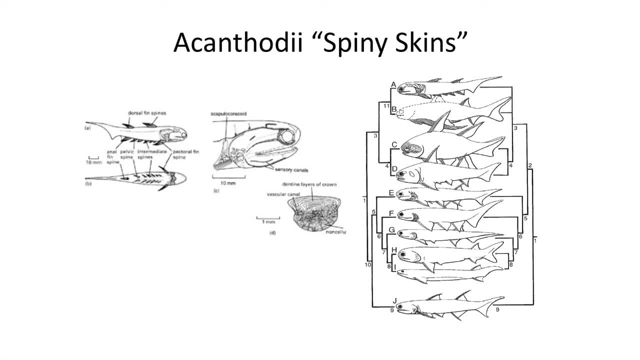 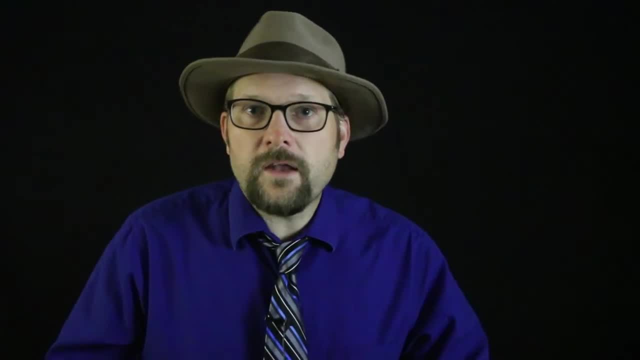 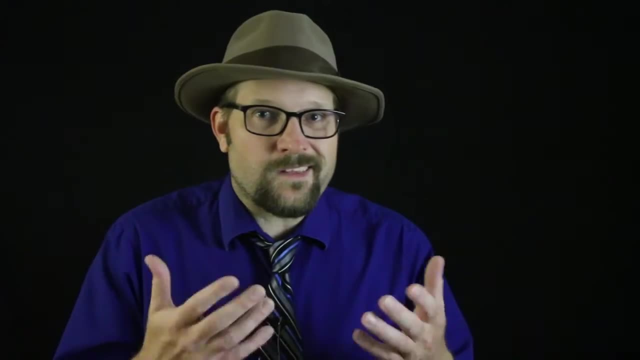 at swimming than the armored plachioderm fish. The gills themselves have gill rakes, a stiff support that is found in bony fish, another more advanced feature, although the cartilaginous neurocranium shares features with chondrichthyans.